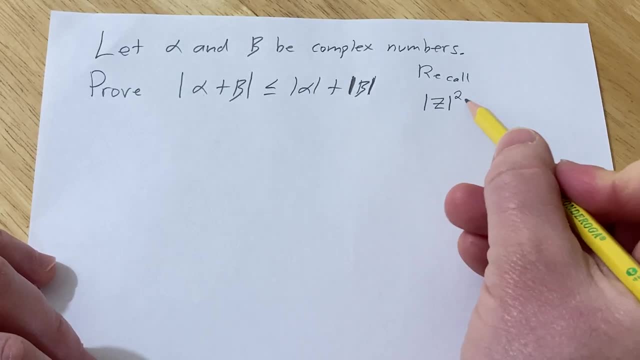 modulus of a complex number and you square it, that's equal to the complex number times its conjugate. So that's one of the things we're going to be using. We're also going to use something that says, if you take the conjugate of the conjugate, you get back what? 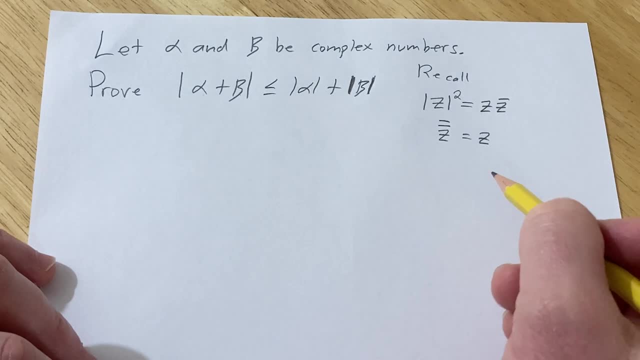 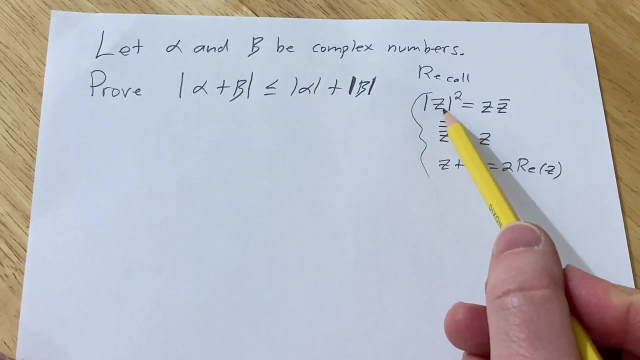 you started, Okay, and we're also going to use something that says, if you add a complex number to its conjugate, you get two times the real part of the complex number, But the key one, the one we're going to use right away, is this one. So, basically, we're going to show that. 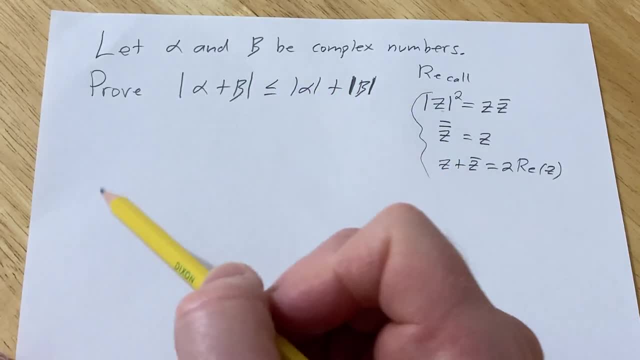 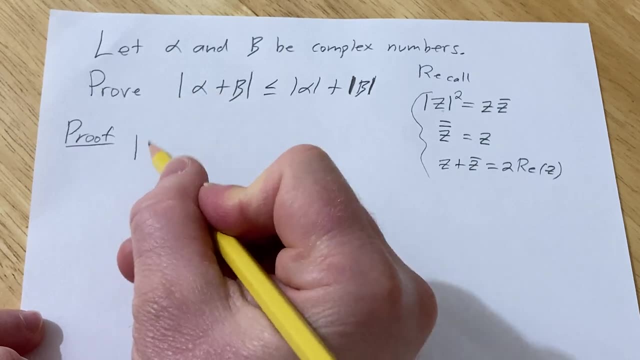 this squared is less than or equal to all of this squared. Okay, so let's start Proof. So we'll start by squaring this: We're going to look at the square of this expression or of this expression, and we're going to look at the square of this expression and. 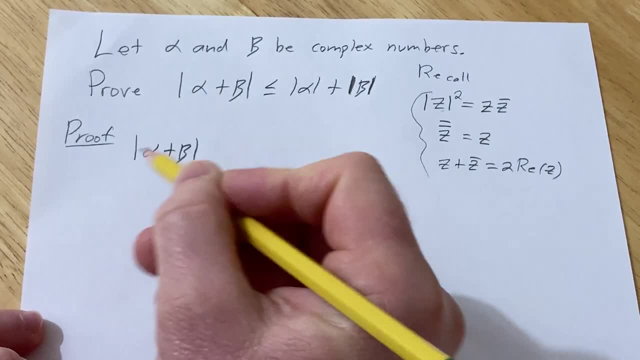 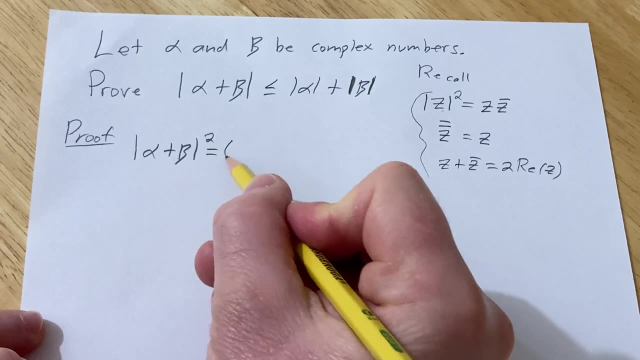 we're going to look at the square of this expression and we're going to look at the number, rather So alpha plus beta, and then take the modulus or absolute value and we're squaring it. So what is this? This is equal to alpha plus beta times the conjugate of: 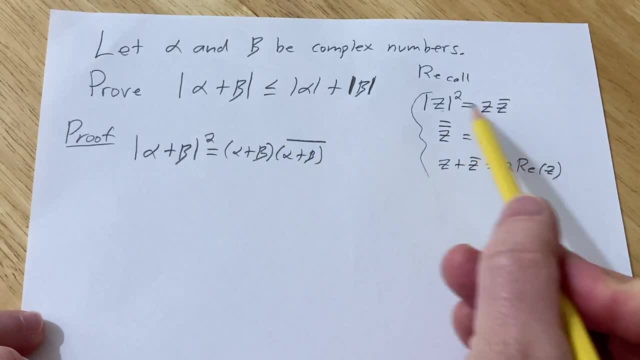 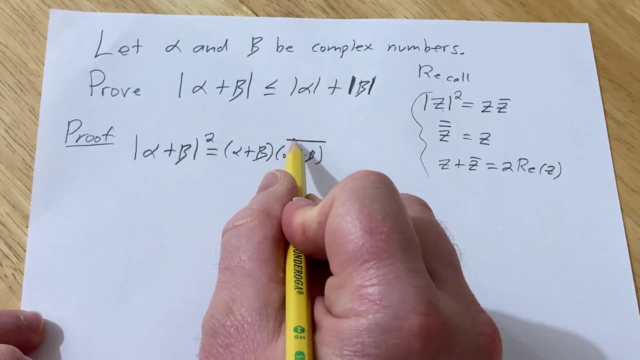 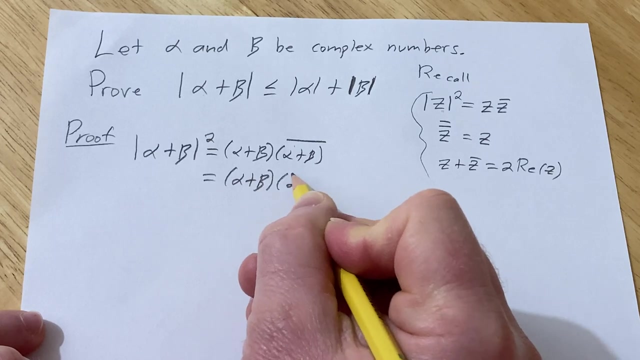 alpha plus beta. That's by this formula here, which I was discussing, So very, very important, very powerful, very useful. The conjugate distributes over addition, so this is going to be alpha plus beta, conjugate of alpha plus conjugate of beta. And now let's just go ahead and multiply this out. 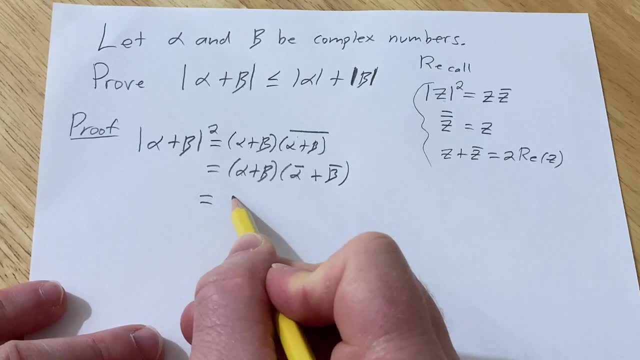 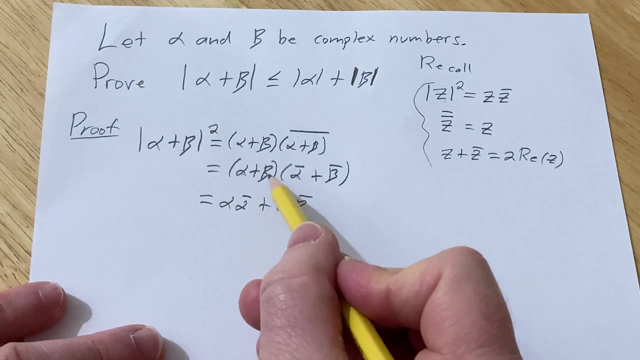 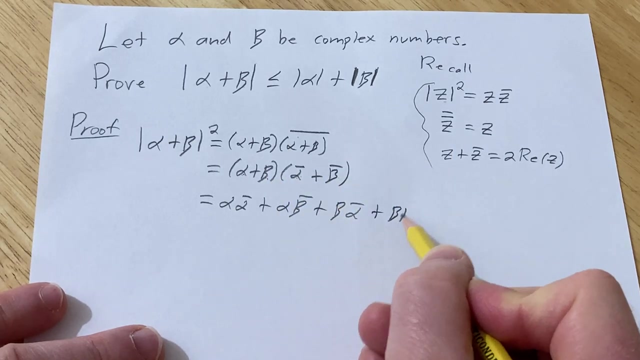 So let's just start with the alpha. So alpha times alpha conjugate is alpha alpha conjugate. Alpha times beta conjugate is alpha beta conjugate. Okay, now the beta. Beta times: alpha conjugate is beta times alpha conjugate. And then beta times: beta conjugate is beta times beta. 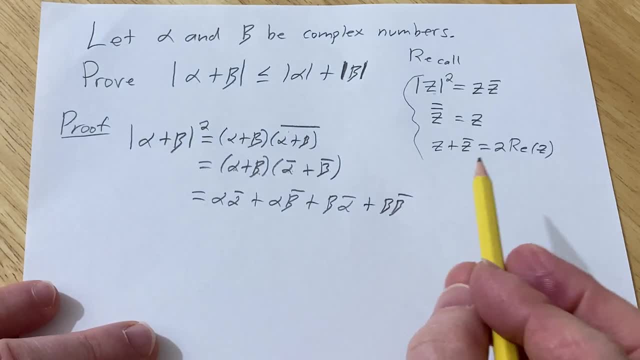 conjugate. So right away, here you see that some of these things are going to be equal to alpha times beta. So right away, you see that some of these things are going to be equal to alpha times beta. So really cool stuff is happening because this key formula which we were talking about is coming up. 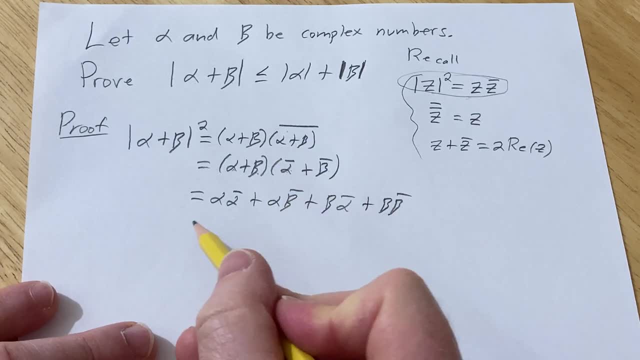 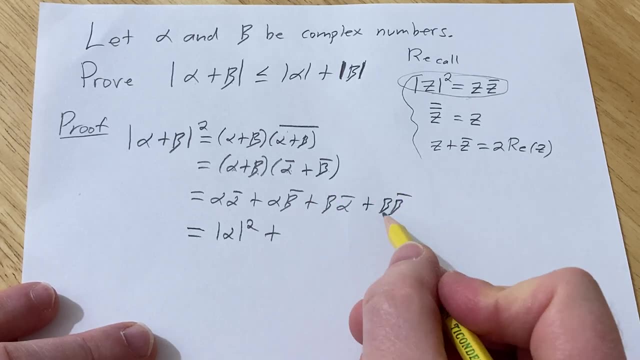 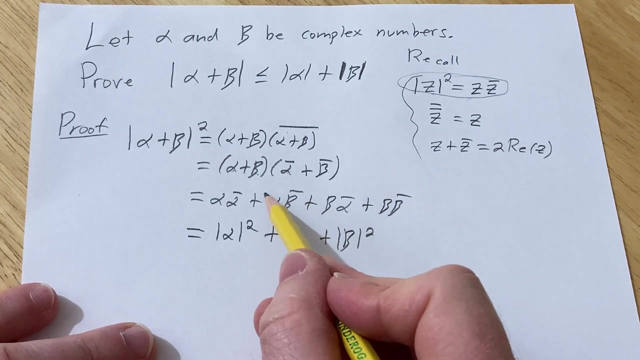 again, right? So right away you can see that this is going to be the modulus of alpha squared and this one over here is going to be the modulus of beta squared. So the issue is: you know what goes here? What can we do with these pieces here? So we're going to try to use this. These look very. 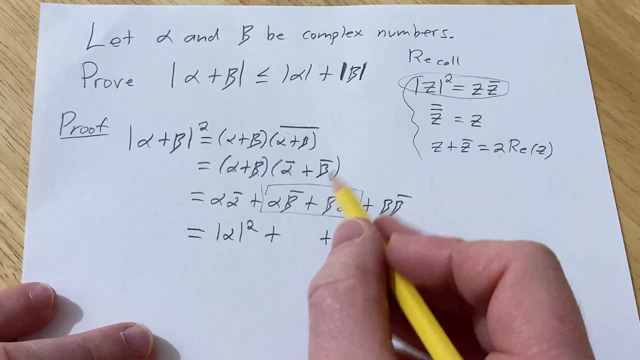 similar. So we're going to try to use this. So we're going to try to use this. So we're going to. The way to figure it out is just to figure it out. So I'm just going to take one of these. I'll take. 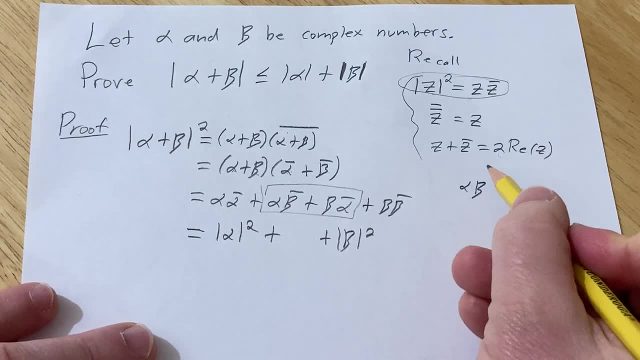 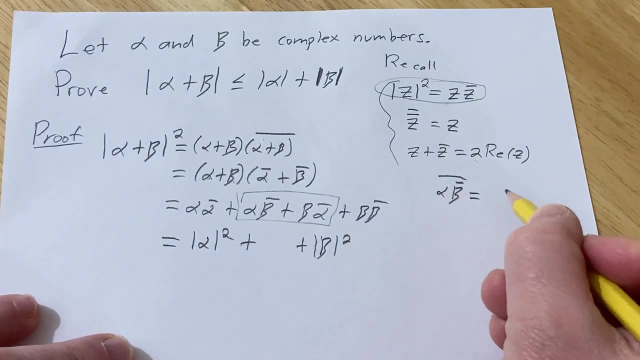 this one. It doesn't matter which one you take. There's multiple ways to do this. Watch this: And if I take the conjugate of this, what is that going to be? Well, the conjugate distributes over the product, So this will be the conjugate of alpha, and then conjugate conjugate, So it's 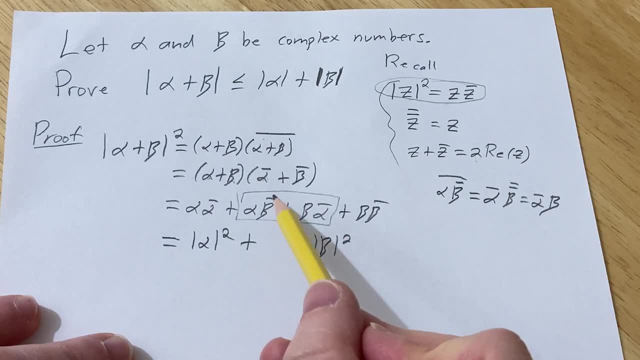 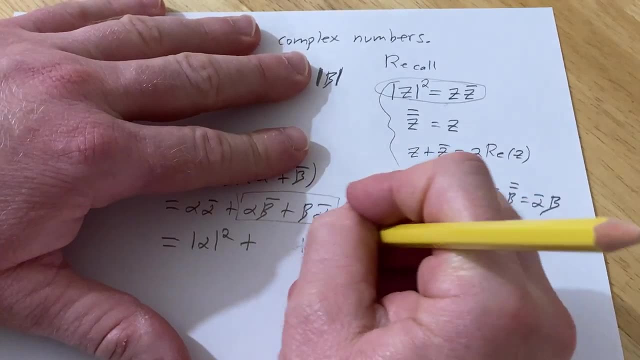 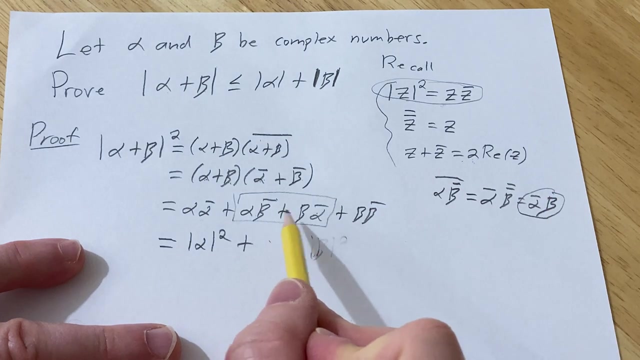 conjugate of alpha beta. Oh, look at that. So the conjugate of this is over here, right? So what we do is we're going to erase this, Okay. so this is equal to okay, which is here. here is equal to the. 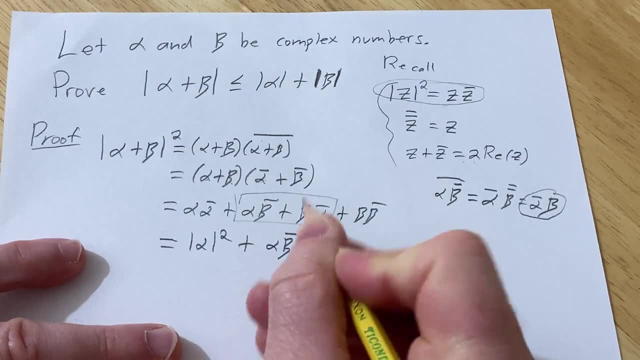 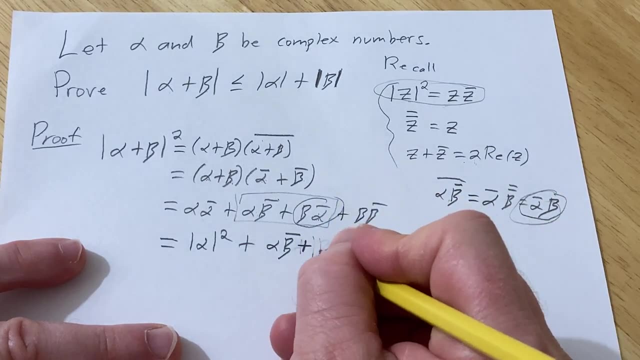 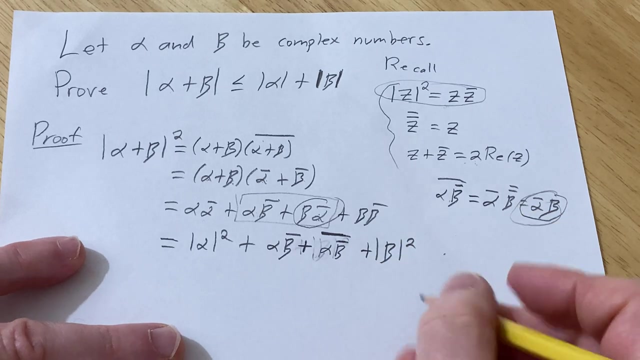 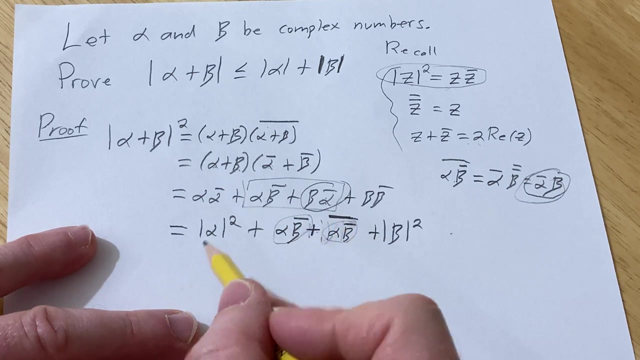 conjugate of this. So I'm going to write this as alpha beta conjugate plus and then we're going to replace this with this. So this is alpha beta conjugate conjugate plus modulus squared. So now what we have here is we have a complex number plus the conjugate of that complex number. 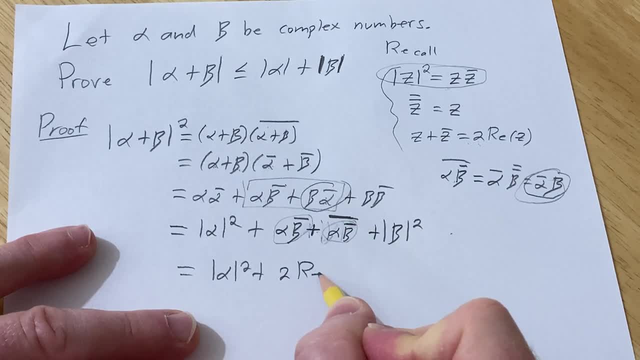 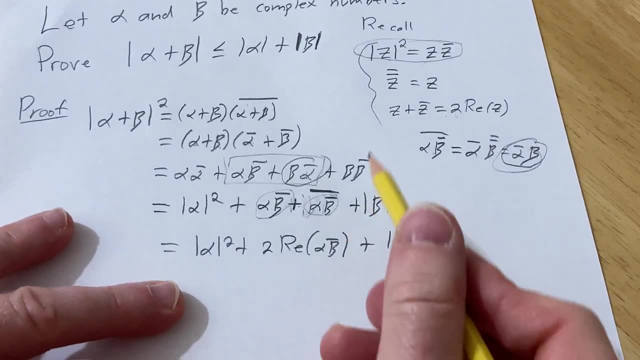 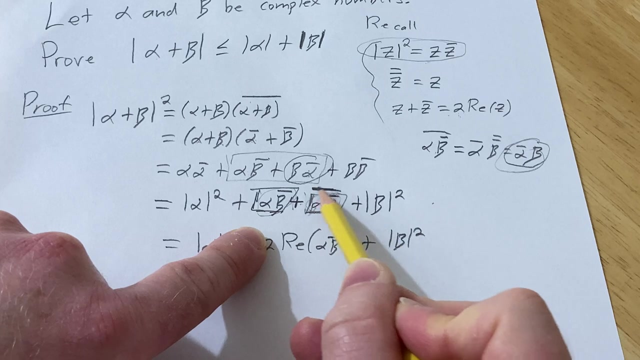 So we know that that's equal to two times the real part of that complex number, And this is probably the trickiest step, I think, in the entire proof right. So again, notice that this number is the same as this number and we just have a conjugate over it. So 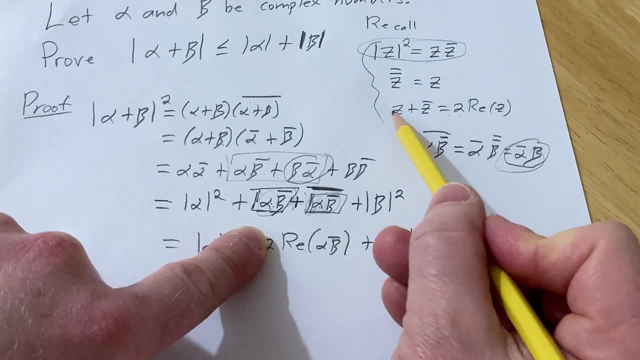 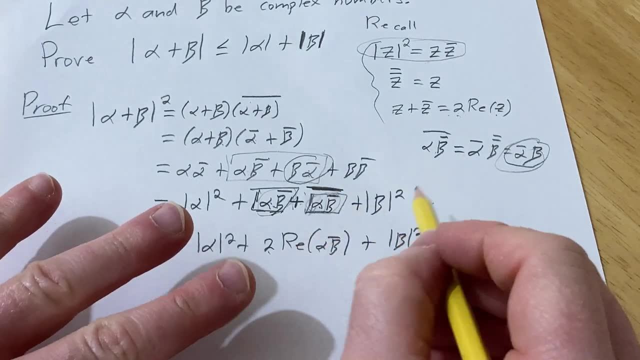 this is your z, z plus z conjugate. Right. Z plus z conjugate is two times the real part of z. Z plus z conjugate is two times the real part of z. By the way, if you instead take the conjugate of, let's say, this one, you know, let's. 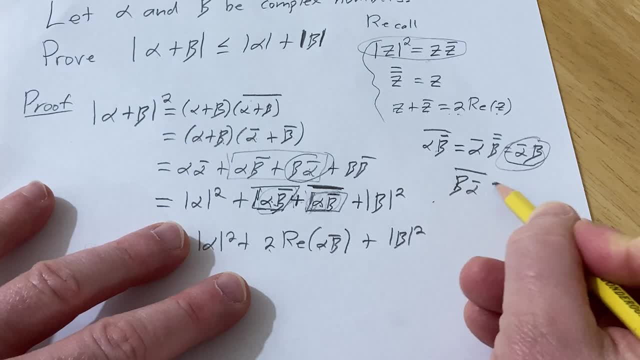 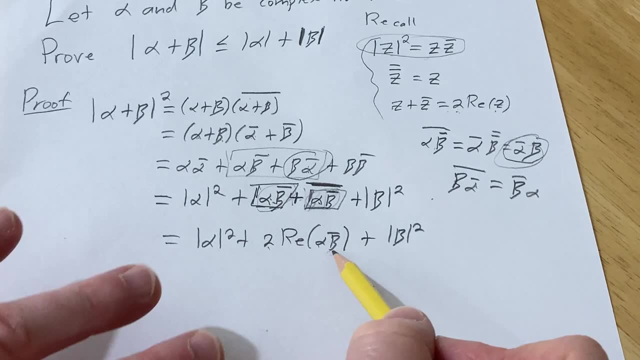 say you had chosen this one instead, that would just be beta conjugate and then conjugate conjugate to alpha, So you would end up with this. So it still works. You get a different complex number here, but it'll still work, Like you could still do the proof Now, something that needs to be. 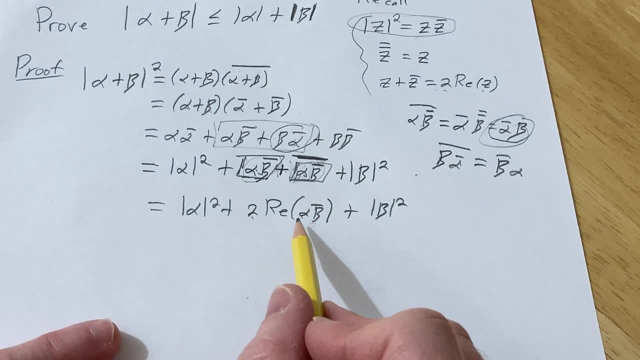 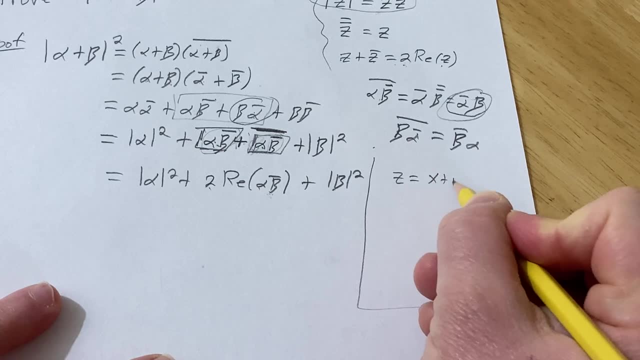 noted here is that we can create an inequality now. So we can create an inequality now and we can create an inequality now with the real part. So if you have, it's just a real here. if you have a complex number, say z equals x plus iy, right, Then the real part of z, that's x, That's equal. 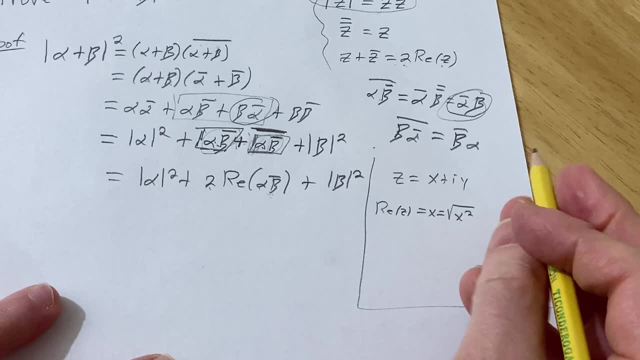 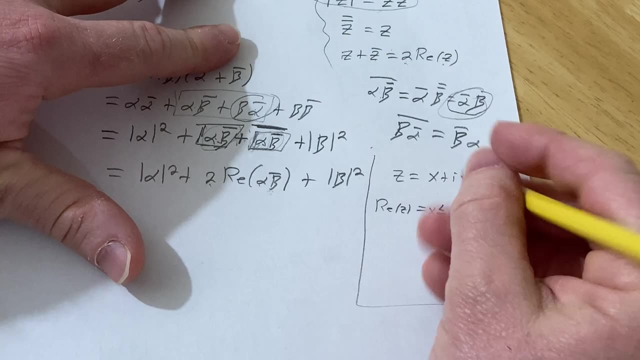 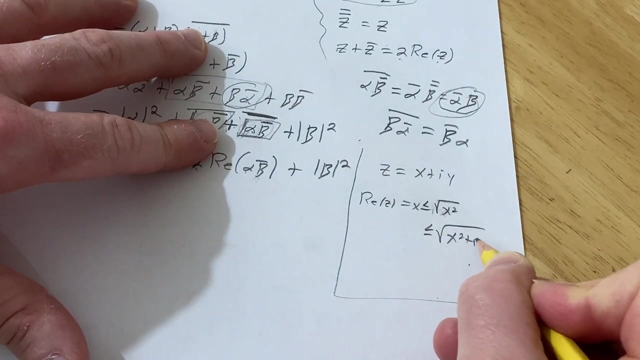 to the square root of x squared, as you know as long as well. actually, it's less than or equal to the square root of x squared right, Because x could be negative here- And that's less than or equal to the square root of x squared plus y squared, which is the 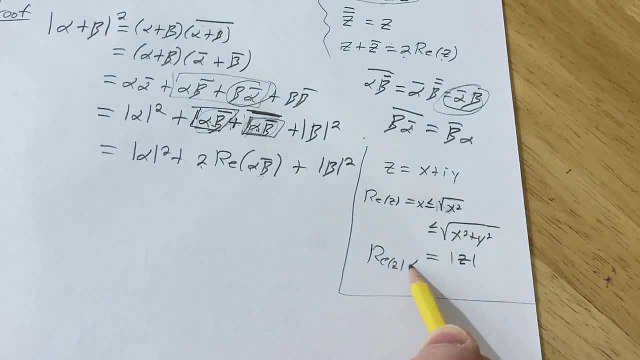 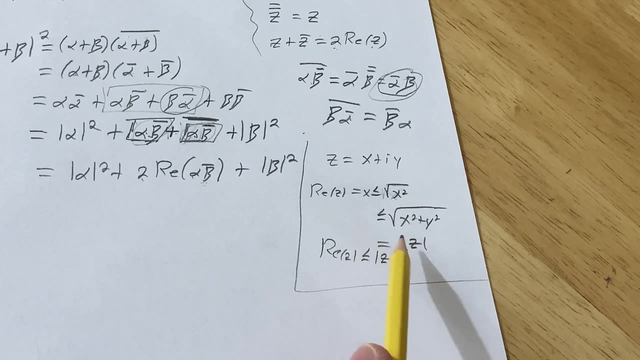 modulus of z. So the real part of a complex number is less than or equal to the modulus of the complex number. okay, Because you can do something like this, all right. So very, very important to note The equality here. would be true if x was non-negative, right, But I didn't want to put. 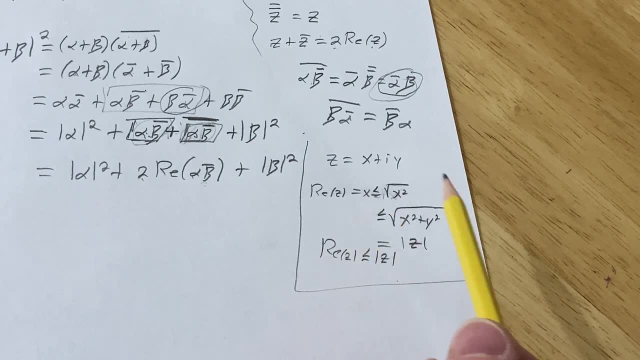 an equals here, because if x is negative, then it's actually going to be less than right, So you do have to be careful there. And then this is obviously true because this is a bigger number. right, You're adding a y squared. 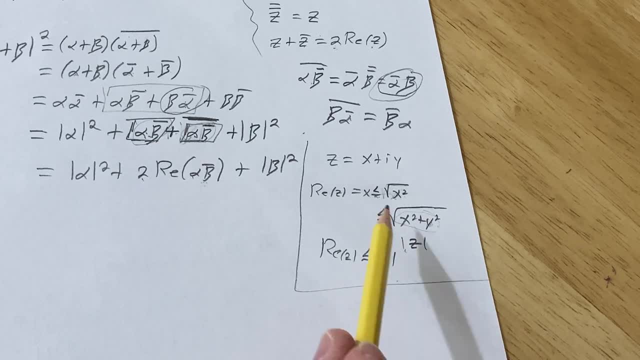 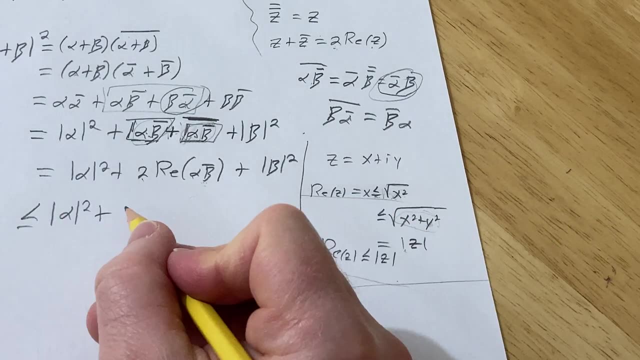 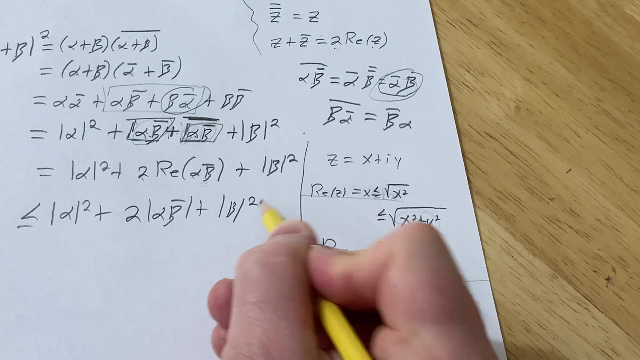 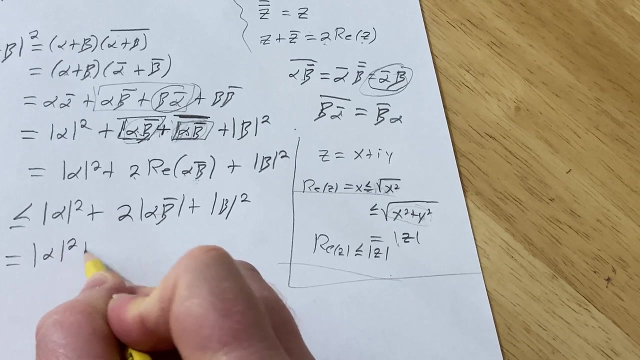 which is also zero or positive, and this is the modulus. So all is good here. So this is going to be less than or equal to the modulus of alpha squared plus two times the modulus of alpha beta conjugate, plus that piece there. All right, so now we can break this up. So this is equal to this. 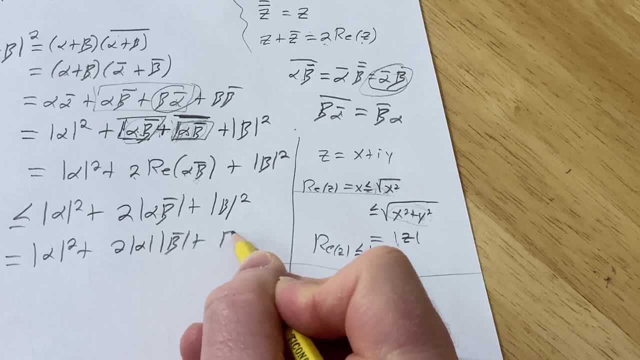 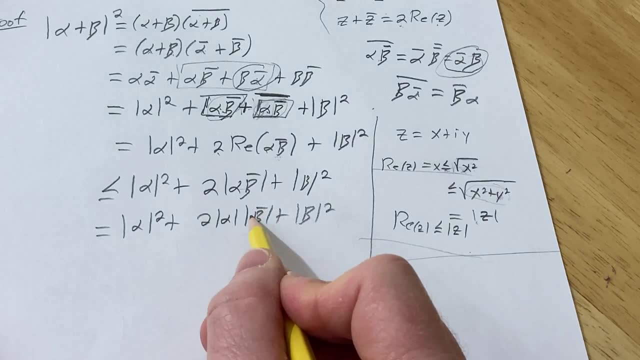 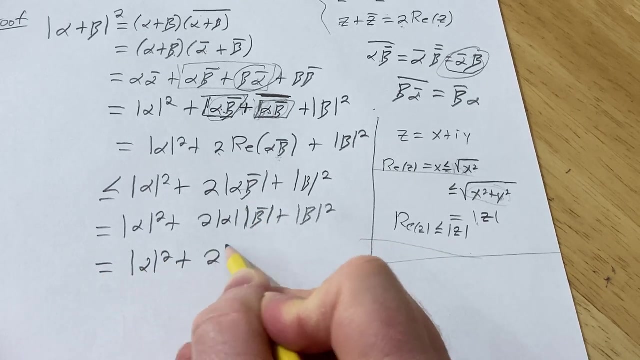 right. You can distribute the modulus over the product And whenever you have the modulus of the conjugate, it's just the modulus of the original complex number. So this is a good proof because it requires that you know like a lot of the basic properties. 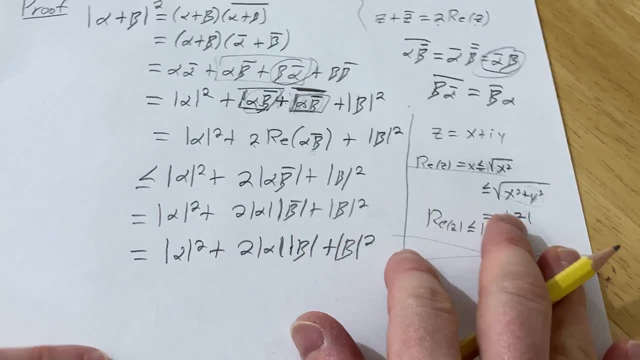 So it's worth like: if you're following this video and something's unclear, it's worth that you go over it on your own. So if you're following this video and something's unclear, it's worth that you go over it on your own. So if you're following this video and something's.